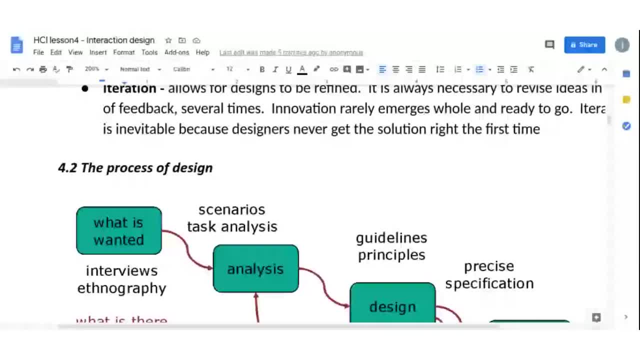 designing for interaction. so you can think of this, like you are deciding the user interface and the user interface. then we say: do prototype. so this is where we are iterating. so we keep here, we, we design something, of course, the prototype design, then we convert it to a prototype, a simple prototype. 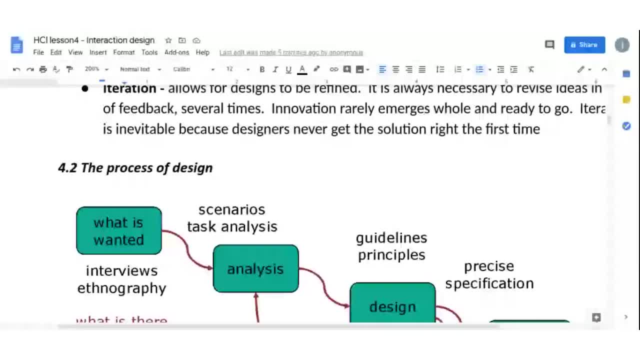 the user uh, work with this prototype and we are observing- or the developers are observing and getting feedback- whether they have managed to get the right thing, uh, that the user can can actually be happy with. so once we do that, we go back to the analysis stage and we we, of course, we correcting 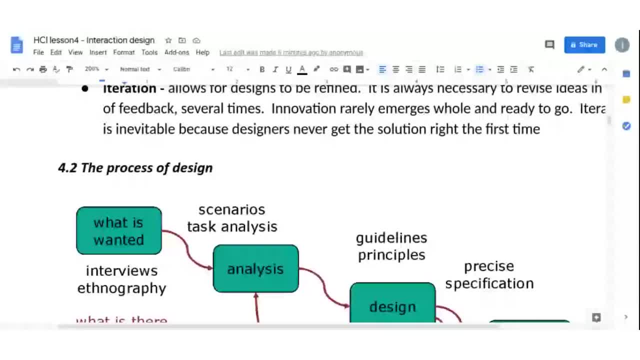 the uh. from the evaluation we are, we are collecting some, some analysis and we are collecting some, some new requirements, so to speak, and so we are analyzing them and also doing the conversion to a technical language and so going on and doing the design again. so we might keep here for a while. 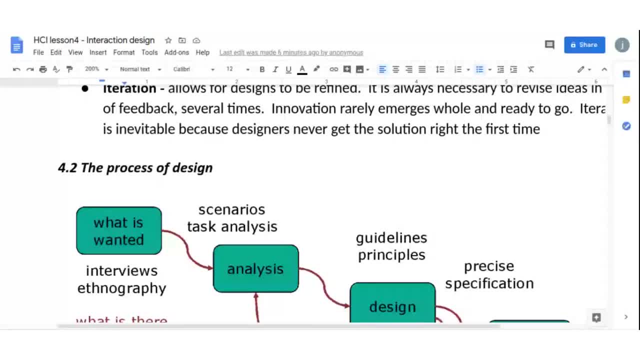 until we feel that the user is satisfied by our design. if the user is satisfied with our design, then now we can go ahead and do the final stages of the final stages of developing whatever we are developing where he is doing now, to employ him and do the deploying. of course, the implement is the developers: build the system and then 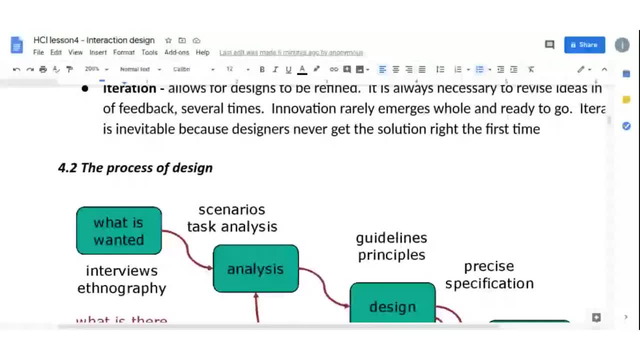 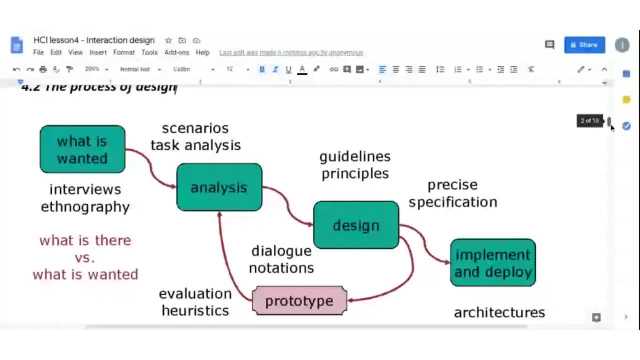 deploys, give it to the user. it is already, uh, no, no more designing now. it is. that is what the user will continue to work with, and so that's just capturing the process, uh, in a diagram form and, of course, as i said, when you look at, this is a resembles very closely, uh, what you've been learning. 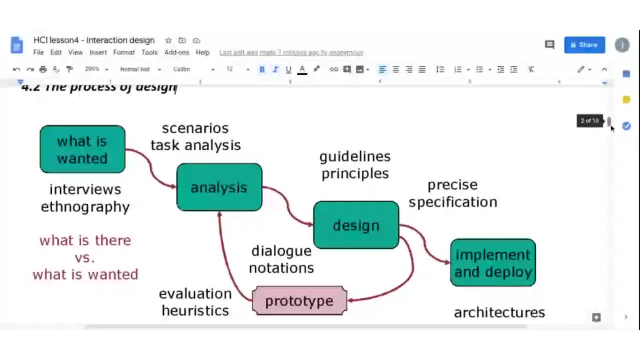 about the sdlc. of course it is known as detailed. i think is a certain living, certain things like. it is not saying how do you test it, but of course, when it comes to a test, our test is here. so, as we do the prototype and let the user, uh, do some, some work with it, that's when we doing. 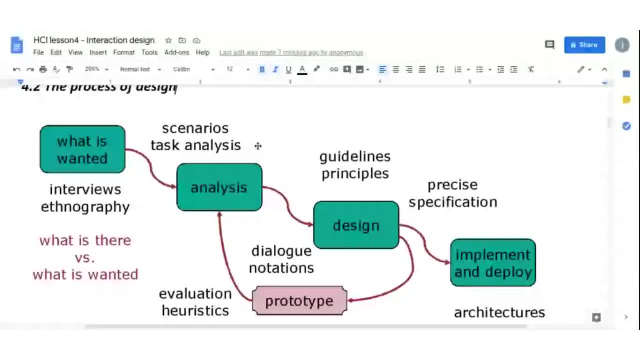 our testing, but of course, in case we don't call it the testing, so of course there's something. uh, terminologies that don't that do not come here, because it's just a part of: uh. sorry for that, so it's just out of um, i think i went down somewhere. 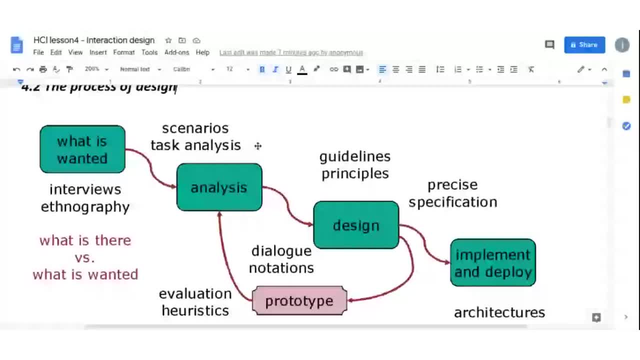 uh. so this is just part of the process dlc, because, uh, here we are focusing more on just uh one, uh part of the the whole development uh, where we are just focusing on the user, the user, what you can call the user interface. all right, so we are focusing just on the user interface. 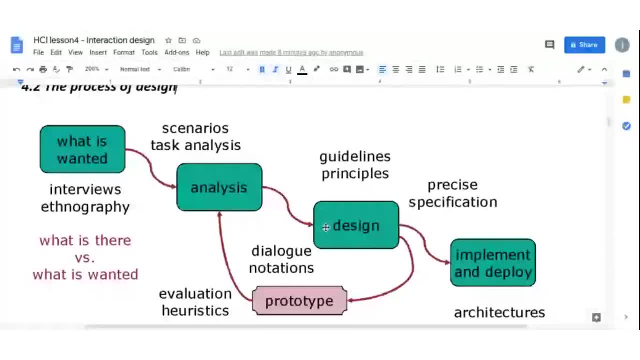 so to speak. uh, so how do we deal with that? so this uh diagram is trying to encourage us what we need to look at and how we can go about it as we try to understand the user and build the right item for interaction, the right user interface. uh for the interaction. 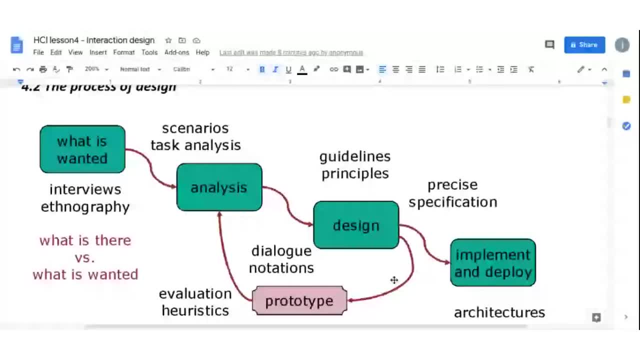 okay, so the, the losses, um, the stages are further down there, uh, which i don't think we'll need to do that together now, uh, are you center design? so what is this center design? uh, so, in this case, when we are designing for the interaction, we emphasize on user center design, or user center interaction design. 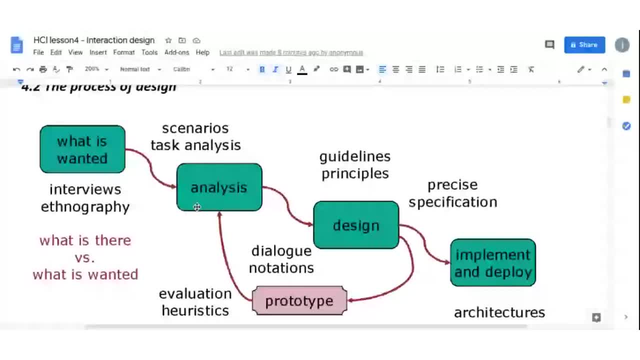 user center design. is a user center design- sorry- is an approach to software development. you set a sign: focus specifically on making products to be usable. okay, the approach: type: client tells- involving users in the design and testing of the system so that their feedback can be obtained. a prototypes i usually employ. 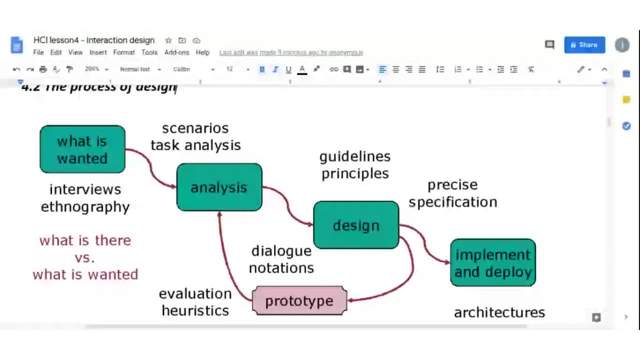 it to do this and designs a modified light of the user feedback. so user center design is a popular user. as much as possible, uh. and of course uh using the prototypes. the prototypes are used so that we can grasp the the the original user, on what we are designing and 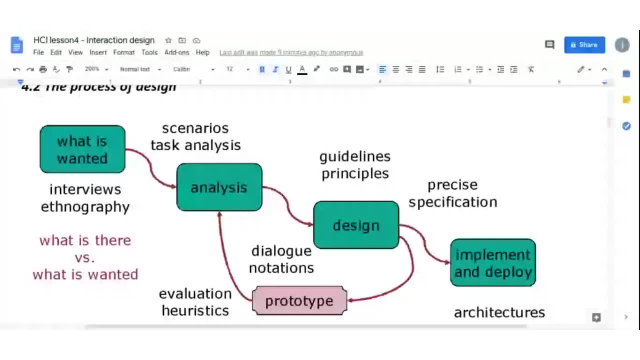 then we get it back to improve, uh, our design. all right. so you could say, initially it may seem that the user center approach to complete cases of their development task due to the need to make identity refinance to their software in light of the user feedback. uh, he sees all. uh, it may look like it's a. 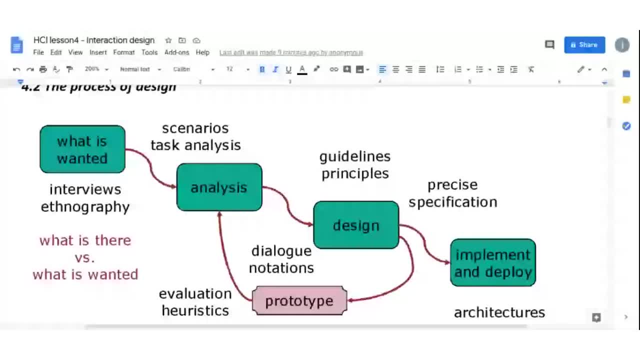 it has more work to the developers. but we always say that, uh, it's better to take a little longer. at that point, uh and uh have the user kind of owning the process and owning the system and also, of course, hopefully also get being happy about what is being designed. then, uh, you know the user and 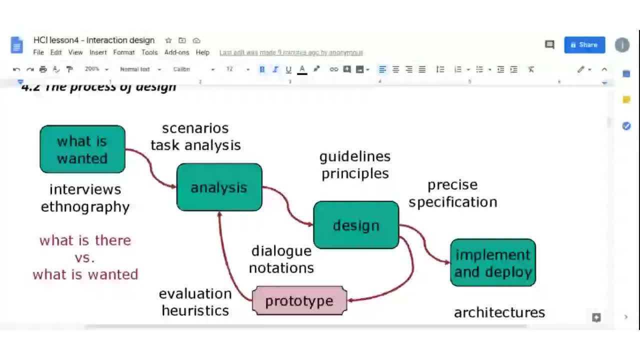 then, at the very end, the user rejects the product. it's better to take some time here, and so, as you move on, the user is already owning the process, we will also own the product and of course, they hopefully uh has shown that, uh, it's happy with what is being decided. so, uh, principles of user. 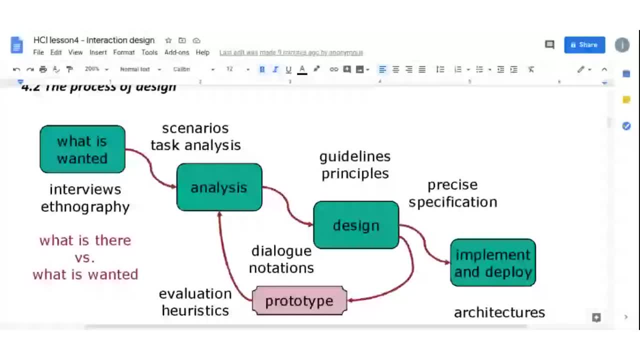 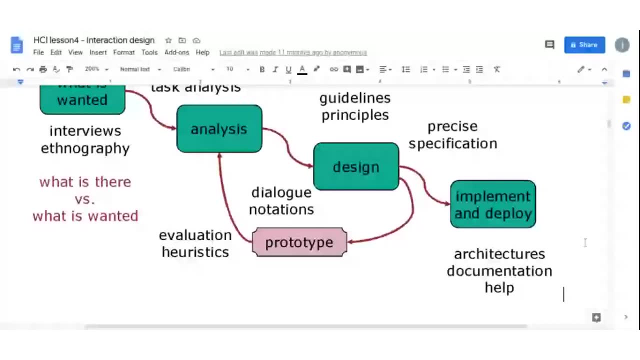 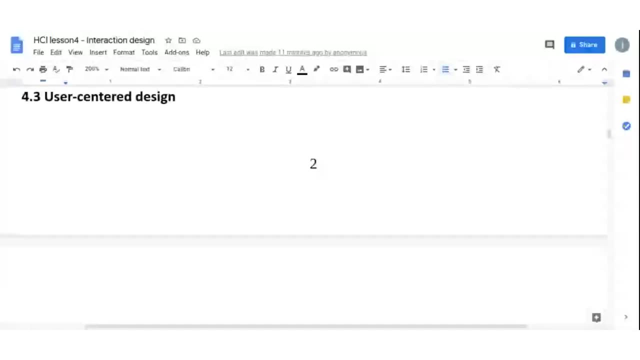 center design is that we focus early in the design process on the users and then measure users reactions and performance uh through various uh approaches. as it suggests, uh use what you call the scenarios, uh use modules, use simulations, use prototypes, uh all these are part of uh capturing. 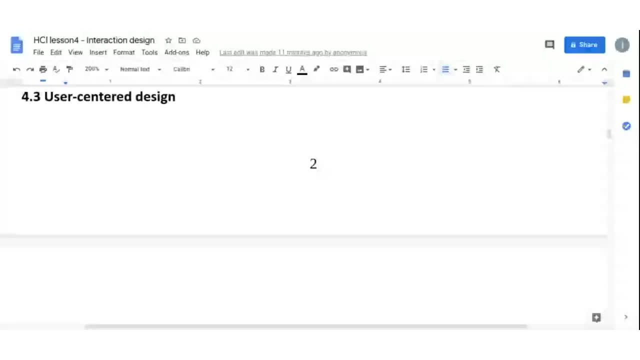 the user reaction. uh, design iteratively. uh, don't move it too fast from one phase to the other, and especially around the analysis and design part. i do iteration. the iteration actually have something to do with continuing to improve the item from the. if you want, you can call the, uh the version, so the, the previous version is improved. 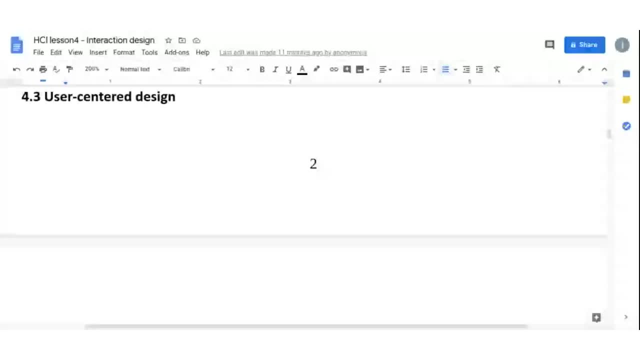 to a new version that one is also improved further is improved further. so education simply means that you are going to improve what was there before, uh, so that is iteration and, uh, of course, repeating a certain process, and of course, the more the focus of the word iteration is improving what was there before, until, of course, you, you get. 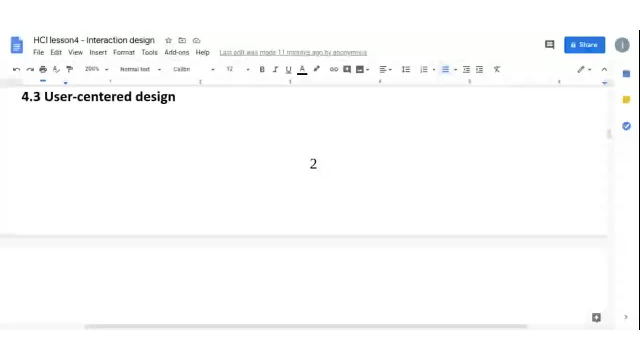 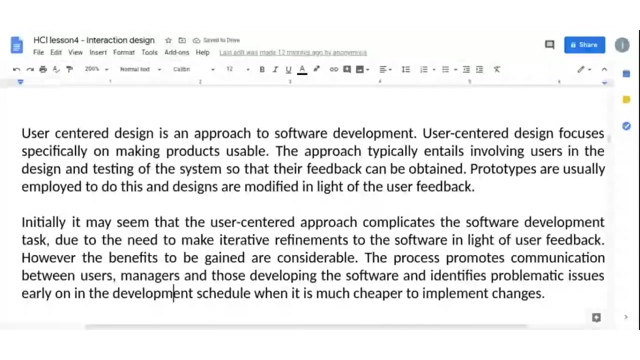 satisfied that everything has been put into uh, into play, so all usability factors must emerge together. is that you are still focusing on usability, usability factors? so are you also seeing that, of course, this is meant to help to improve the usability as much as possible? and so, as we said, this is still a software development and so it is still based. 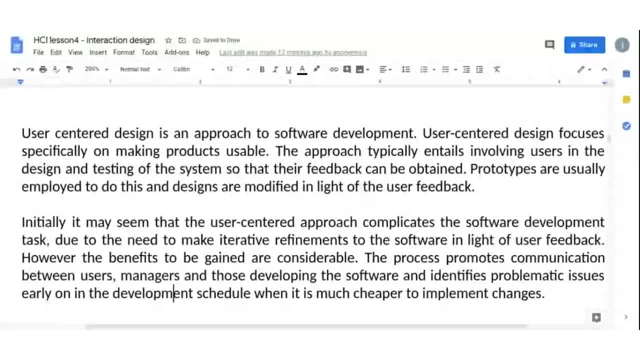 on software development life cycle or system development cycle, and so we talk about the models. i don't intend to talk about the models, but this is already captured from my previous statements- uh that we're still following uh the uh concept of, uh the software development lifestyle. you know the waterfall model, of course. 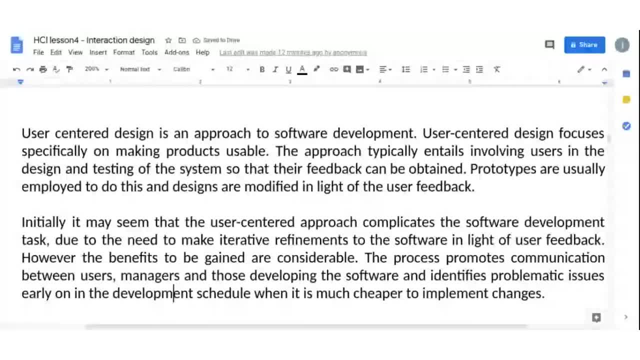 here. now it's different. so we're also asking ourselves what, oh, among us all these software development models, which one is would be, would uh be like the best to capture this concept of user-centered design? and so, of course, there are some which uh would be very close to that. 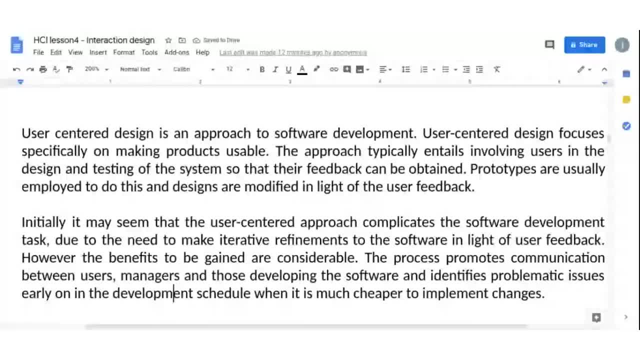 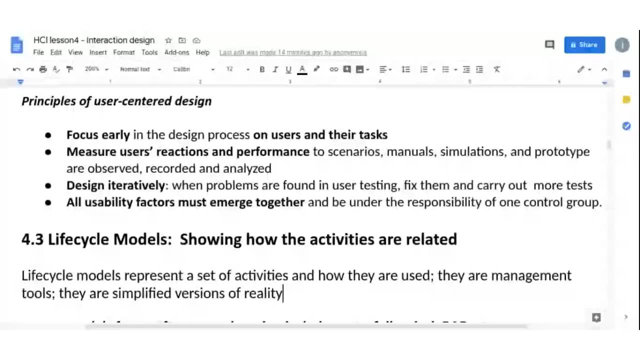 but we have also others that are very far from the concept of user-centered design. well, uh, but uh, this uh subsection here uh tries to discuss a bit of uh these life cycle models, which you already are aware of. so uh just mentioning in passing, without uh taking any: 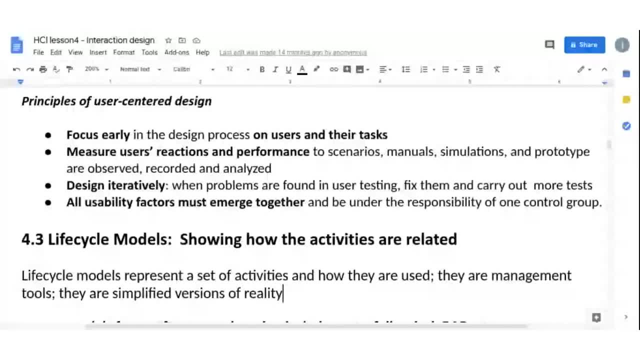 time to do the uh the study there. but of course for you is a very, very important that you make sure that you review your uh understanding uh of the various uh sdlc models, that are, the water forward model uh and others, but the one which approaches because a user center design of. 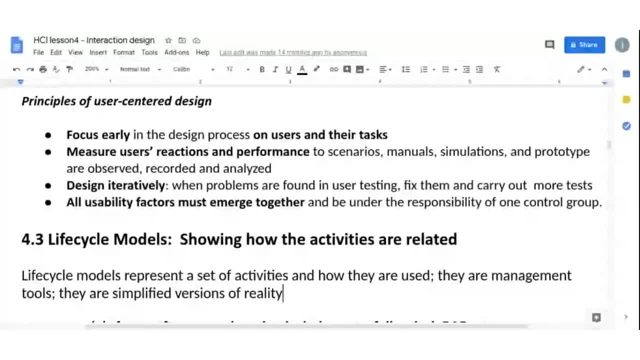 course are those that incorporate uh prototyping and of course we have a number that uh incorporate prototyping, including uh the spiral model. uh, if you can remember, the spiral model has some prototype part where prototyping is done and also uh keeps on improving. you know the rate is doing like a circular thing. uh supposed to be improving. 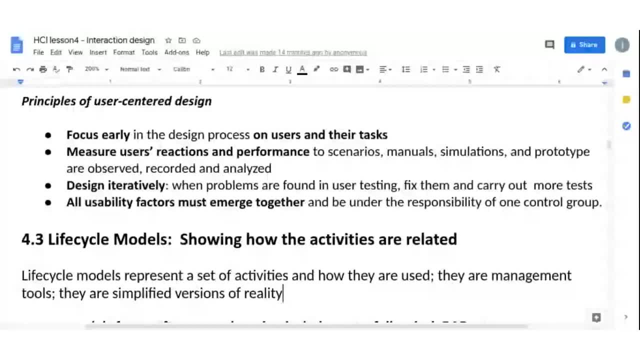 things as it does, as the moving circles are, you know, they're supposed to be improving, uh, and the. you know the, the, the previous design, uh, then a rapid application development is also prototyping, uh, so, and it talks about the various types of prototyping, um, but of course it also involves the. 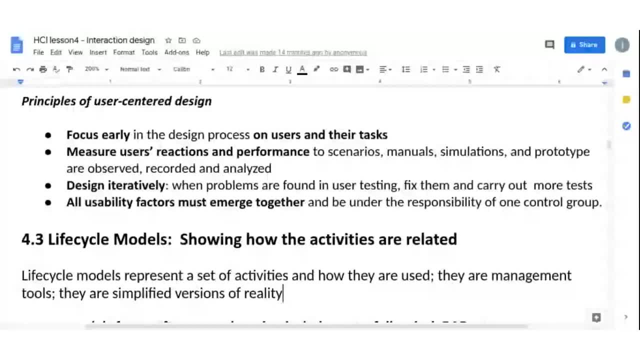 so it's so. the issue here is improving the user and also doing the iteration and creating prototyping. so those are the models that can be used in doing the user-centered design in hci. there is one another uh, more uh focused uh including this one called there the star model. so there's one called the star. 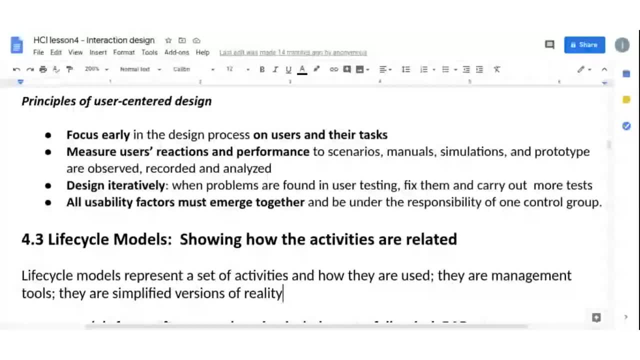 model and the star model uh is based on the fact that uh- and this is a diagram for the for the star model uh- unfortunately, it said to be on whether it will allow us uh to reduce it. unfortunately, uh, sometimes it's a system does not always go very easily. 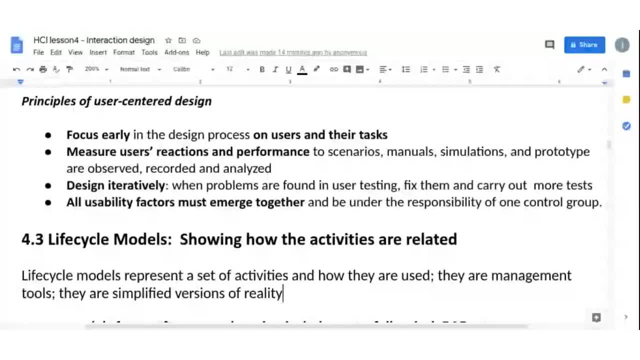 when you try to make changes. let's see whether you can have it fit a little more on our, so you can see the whole diagram on our screen. uh, so that's a well what? uh for not whatever, but the star, the star model. so this is an addition now to what you already have. 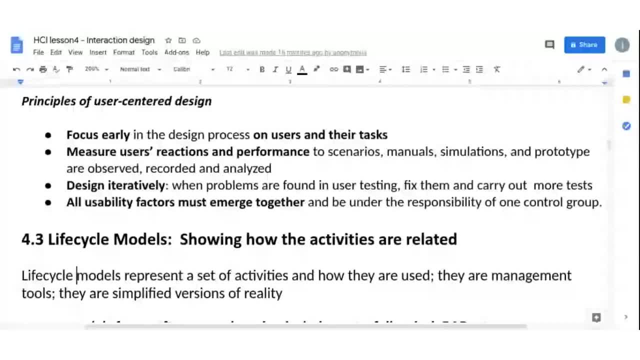 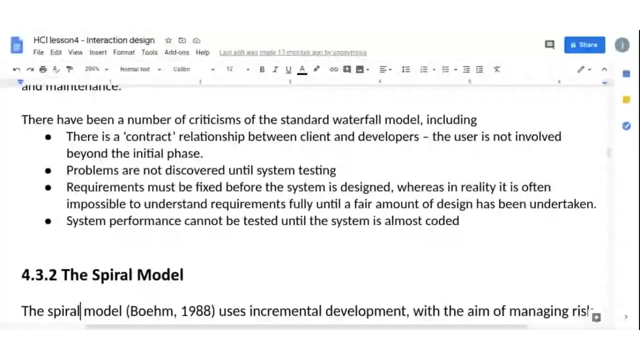 so when it comes to interaction design, we also have a model called the star model. so the star model of course, looks more like uh in a networking topology where we have a withdrawal uh, some middle device. of course is not a device, is just a representation of what is happening. so it's. 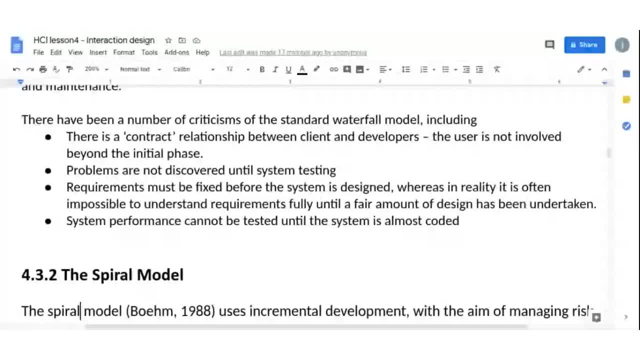 standing in the middle there then, surrounded, you can see some of these words that make sense from development models. so we have uh cause. it is not a organized in any order, but you can recall some of the concepts, like requirements, requirements, so you go out there and you gather requirements, you do the analysis, so you do the. 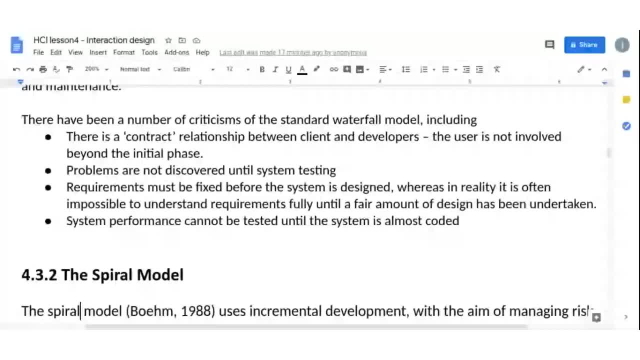 analysis and, of course, you do the design. do the design here, but you also incorporate prototyping, because it's now user-centered design. you incorporate a prototyping and, of course, once everything is ready, after the design is good, then you do the implementation. so the same terminologies, but they're not in any order and what it tells us is that: 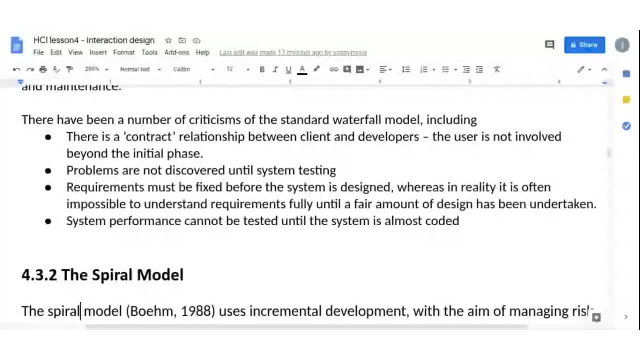 when we are doing the user center design and then our our. the activities that we are going to do do not follow any particular order. what is important is to catch the user, the user's reaction and the needs and the requirements. that's what is important, and so 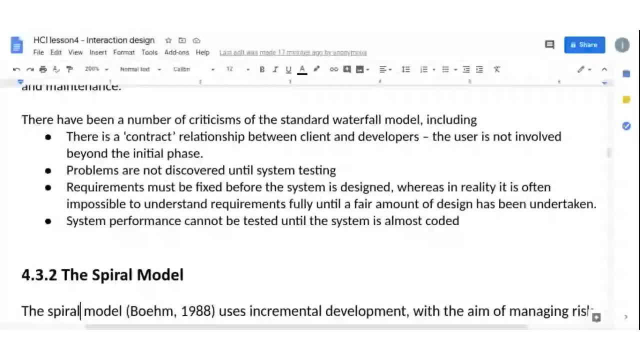 we can keep on going around and around, and. but then the importance of having the evaluation in the mid row is to say that this is very, very key. and of course, the evaluation is done with the user, uh, practicing with the prototypes, uh, so, but it's like everything we do, you always do a testing. 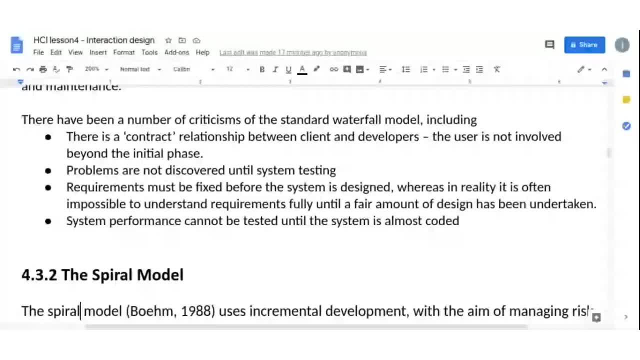 with a user. so, whether you are doing the analysis, you test with the user. uh, talk to you about that. let the user be involved as much as possible through the development process. uh, so of course, the requirements is the obvious, because that when you interact with the user, but again you are keeping on uh testing whether you, uh you managed to capture the users. 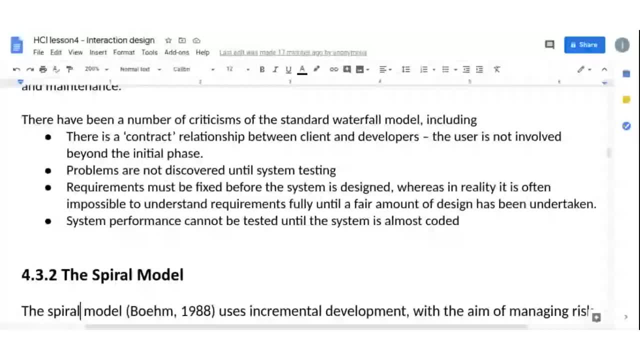 of feelings about the system. so this is called the star model for user-centered design and it puts the uh- what you're calling evaluation- here in the middle to say that for every phase you keep on evaluating, so don't like the waterfall which the user is uh is involved only at the 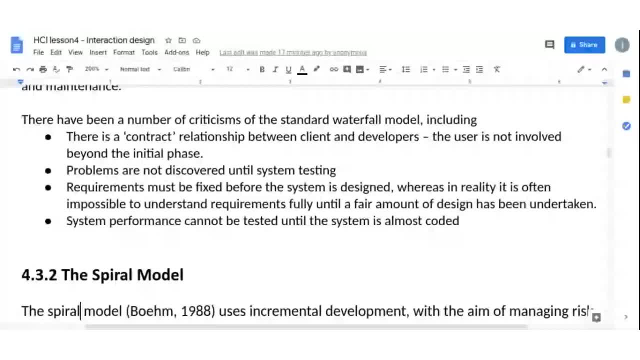 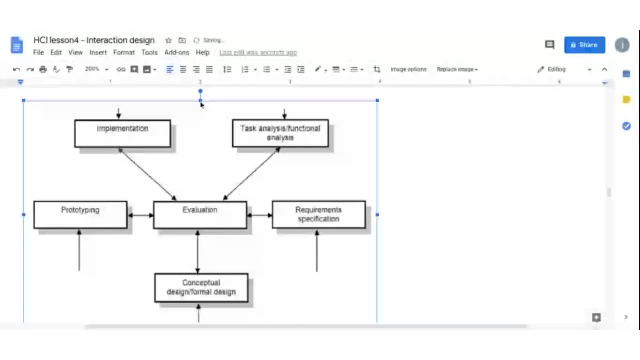 beginning. then it starts moving down and no, the user doesn't have any role to play in those phases, until at the very end, where now the user is brought the item and then they might find that it does not help them. so the best thing is a keep the 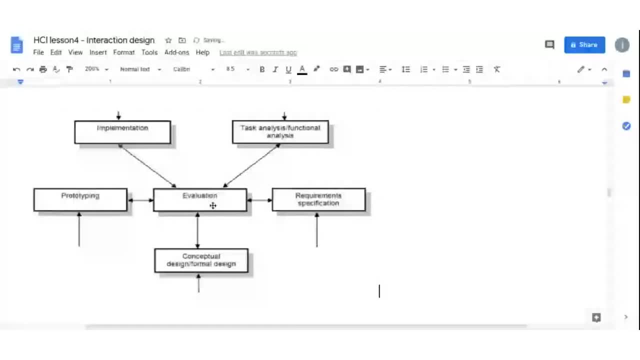 process. uh, let the user test the systems, especially the, the at the design level. let the user giving his or her feedback about the design, and that way you are able to move with the user and come up with something that you know that the user would find useful. so the star. 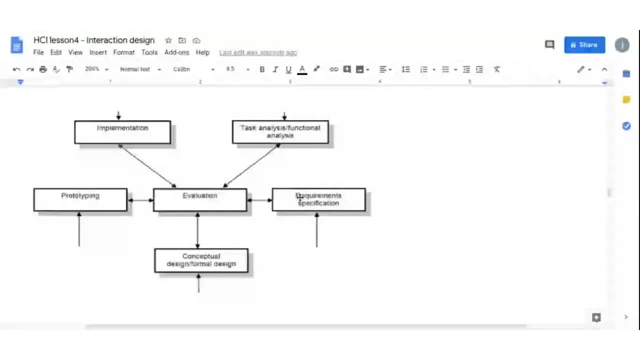 model. so another one, which is a more focused on the user center design, is a, the concept of the usability engineering uh life cycle. so this is also a model, although it does not have a clear diagram uh about it. this is more explained in text. user, we call it a usability hearing ue. 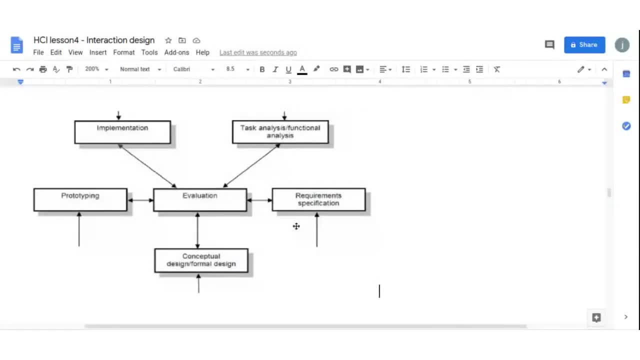 a systematic approach to making software easier to use for the individuals who actually use it to get their work done. it is an approach to the development of software and systems which involve user participation from the outset and guarantees the usefulness of the product through the use of a usability specification. 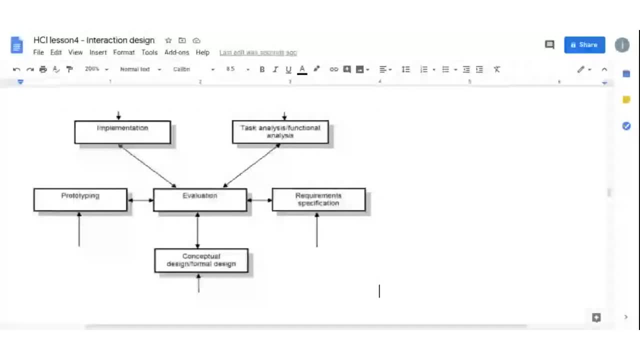 sorry, let me just move this. uh, so, um, okay, so let me read that statement. it is an approach to the development of the software and systems which involves user participation from the outside and guarantees the use of the usefulness of product through the use of usability, of a usability specification and metrics. ue, in short. ue thus refers to the entire. 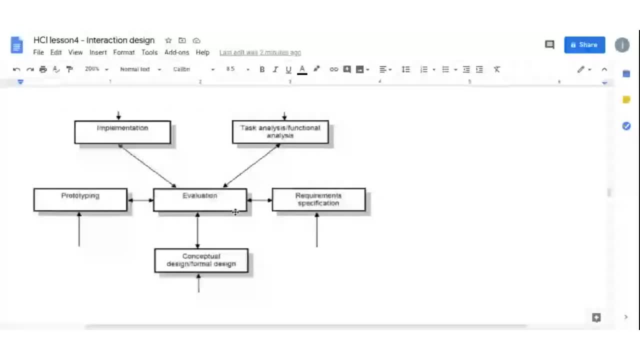 process of producing usable software products, from requirements gathering to installation. ue is based on user-centered design, in short, ucd approach to analysis and design. sorry, let me just answer. uh, yes, uh, yes, amaya, sorry i have to. yes, A part of a self-discipline. Uh, yes, sorry, I'm in the middle of a class. can i call you later? 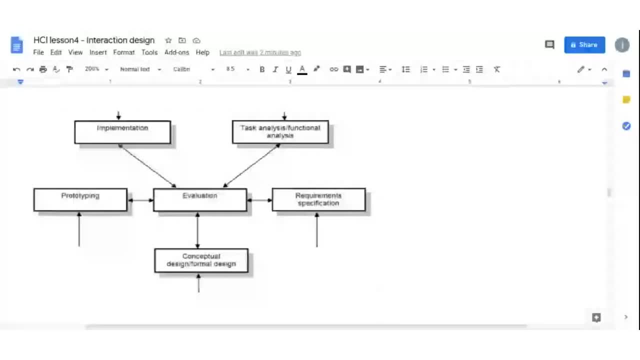 Sorry, I am in the middle of a class. can i call you later The Uh? sorry for that. so, uh, this is another user-centered uh approach, or like it's another uh kind of a model. so this one doesn't have a diagram. of course there's some people do try to. 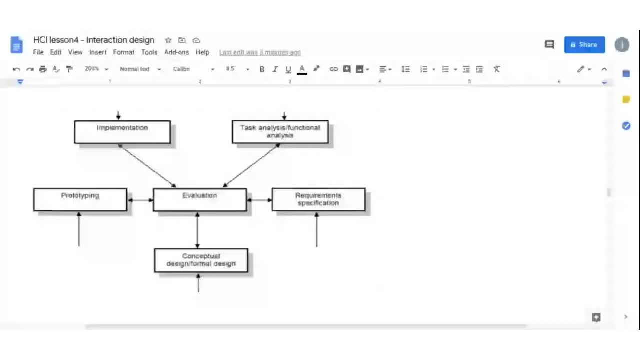 come up with a diagram, but, uh, it is mainly user-centered approach and that is mainly describing text and it is called the usability engineering life cycle and it the way it is it expresses the whole process is explained in this particular table. unfortunately, we may not be able to see the table on the online because it covers quite a large section. 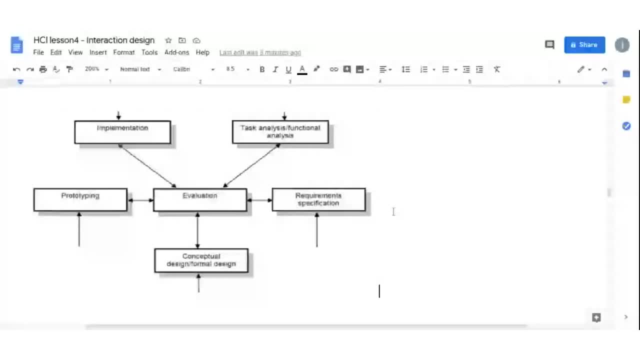 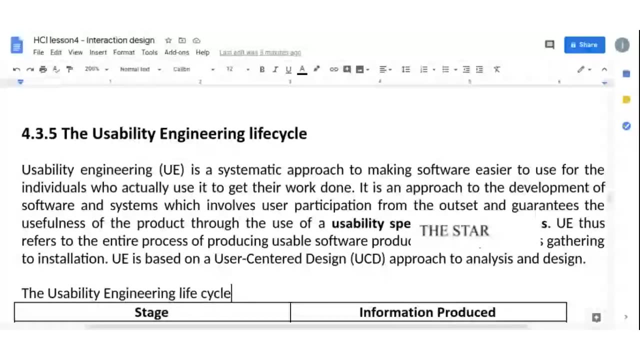 but let's see we can fit it down here and let's see whether it is able to show on one. well, it is a huge table but at least you can see a bit of it. so it's related in life cycle. so some of the stages, of course, because stages uh, although 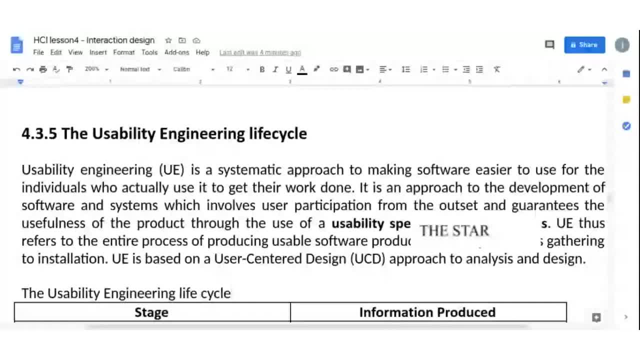 they are not. every research says that they are more like just activities that happen, know the user and know the task, user requirement capture, settling, setting usability goals, etc, etc. and, of course, explain what exactly happens at that particular stage. so when we say no user, we are trying to understand. 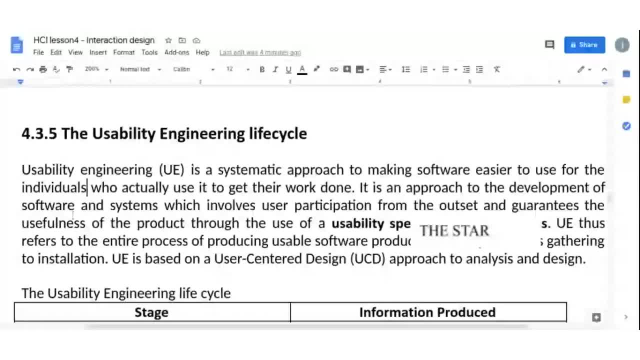 so we go beyond just collecting user requirements, but we also get to know the user and the type of work this user will be using. of course, if it's a computer, what, uh, what type of an environment, the use or whatever the software we are developing? and again, i need to also, i like that. 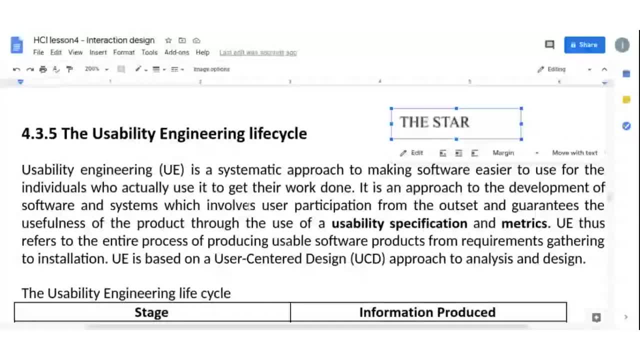 this concept of user-centered design is not just for uh, for user interface, but it can also be applied across the all the, you know the whole phase of all the phases of a complete uh software. so it is not just for the user interface, or except that this point our emphasis is, so the 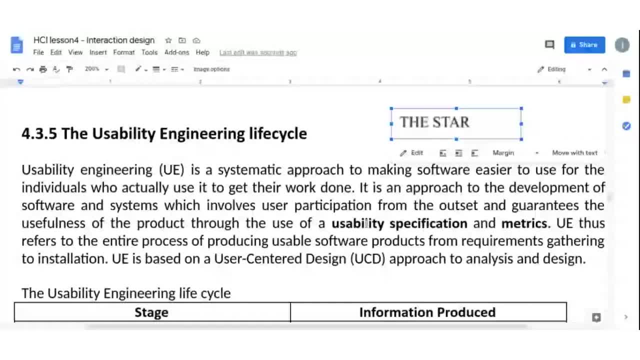 user interface is the whole concept of interaction, and so you will let a look at this: the user engineering, uh, usability engineering, stability engineering, or ue. so that's a another approach, uh, that tries to capture uh, what uh a user center design should incorporate. uh, now, uh, we talked about 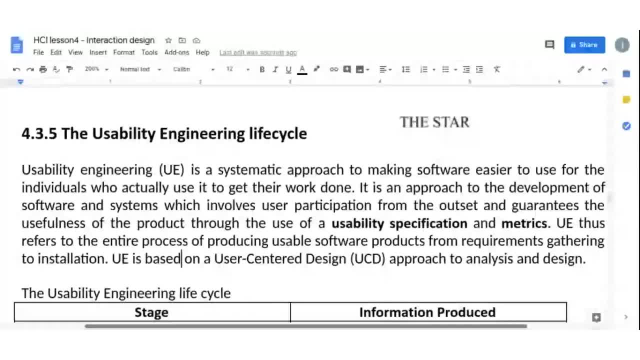 uh, prototyping. so all the software's, the software models that incorporate prototyping. they are good, not all, of course, but most of them are good for user center design because with the prototyping, in most cases the prototyping is always evaluated with the user and so it talks about. so this: 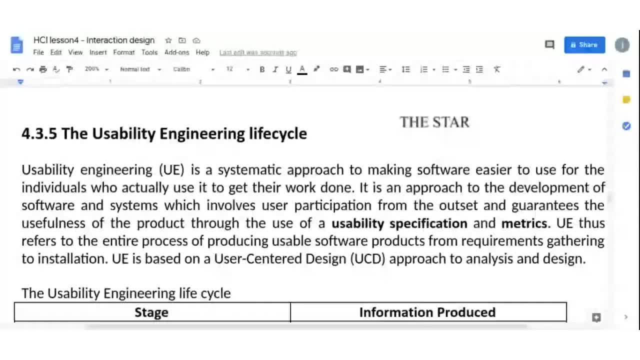 document has a bit of explanations about prototypes and, uh, so what are the type of prototypes you need to create? so we have two types of prototypes: low fidelity prototypes and high fidelity prototypes. so the high, the low fidelity prototypes are those which do not require you to create a kind of you. 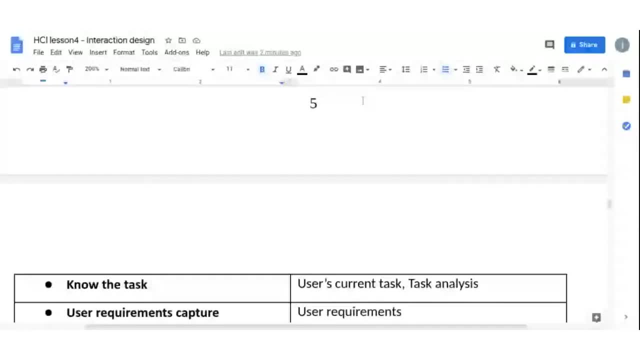 know, um, uh, what we are calling down the interactive system. so these are just like uh designing, just on paper, uh, just simple things, uh doing some uh what we are calling role playing, etc. so those are low fidelity prototypes. but the high fidelity prototypes, of course, is a software, is a kind. 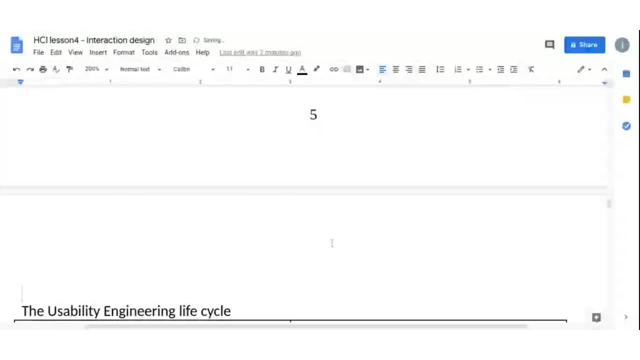 something that is a little more interactive, uh, most like a basic software, uh, that is a trying to present an interaction, uh platform for the user. so, low fidelity prototypes versus high fidelity prototypes, uh. so, as i said, there is a document also gives the various types of prototyping, which you already are aware. 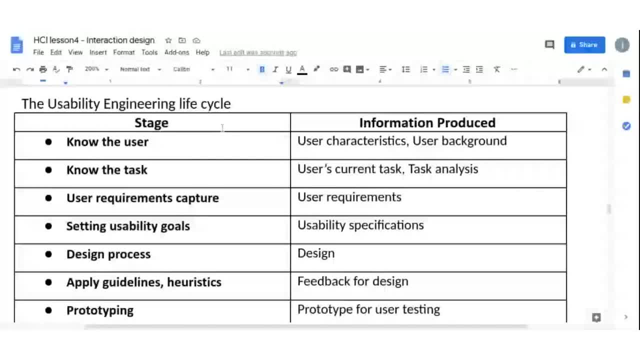 evolutionary prototyping- draw away, prototyping. and evolutionary, you know, incremental prototyping, incremental, so evolution, evolutionally- draw away. and incremental, uh, prototyping, uh. so the other important concept in the user center design is something called the contextual design. contextual design is the design of the user center design and the design of the user center design. 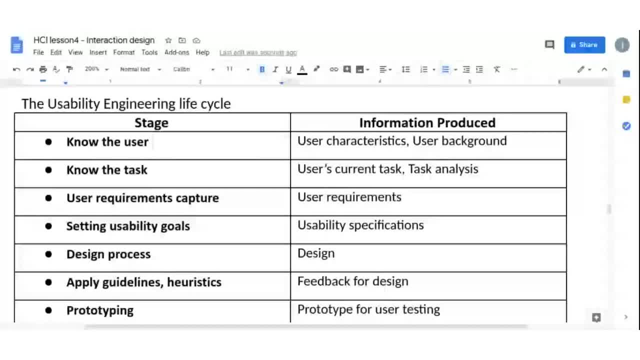 and the design of the user center design. now, the focus on this is that it's good to also capture the requirements, capture the, the user requirements, by visiting the user at the, the environment where they will be using the, the product, and you get to uh feel that the, the and 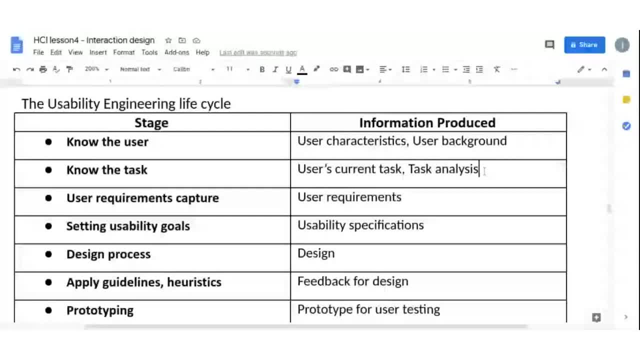 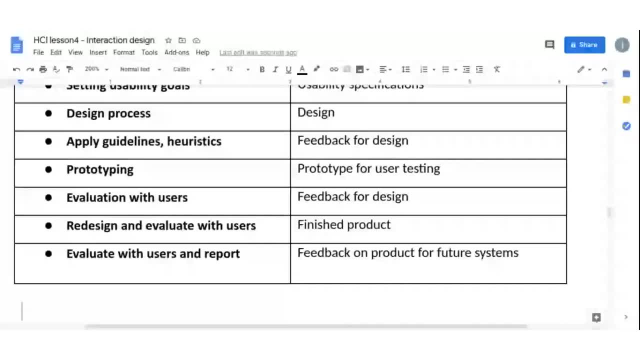 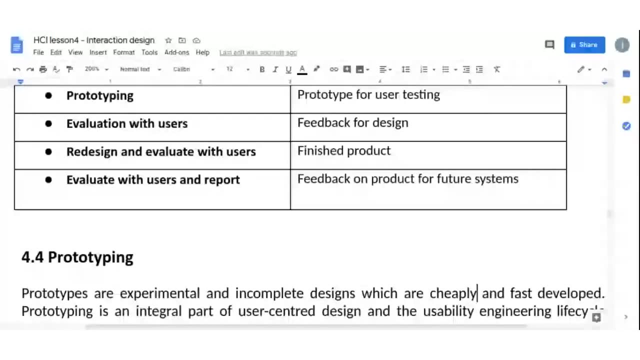 of course, also to see, uh, the way the this particular user does their work, their day-to-day work. that might be very helpful in coming up with a design that would be useful to this particular user. so contextual design focuses on going to what we're calling to go to the field. it's actually very much similar to what we now. if you think about a. 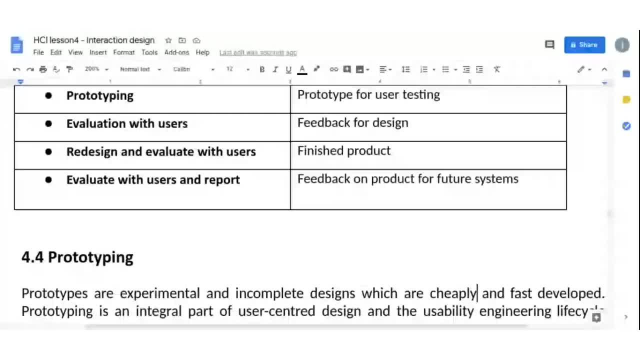 research. when the research, we say the various ways of collecting data, and one of them is called observation. so this is a just another way of talking about um uh observation, the, the, the memory observation, where you go and you observe the user at their place of work and you capture that by just. 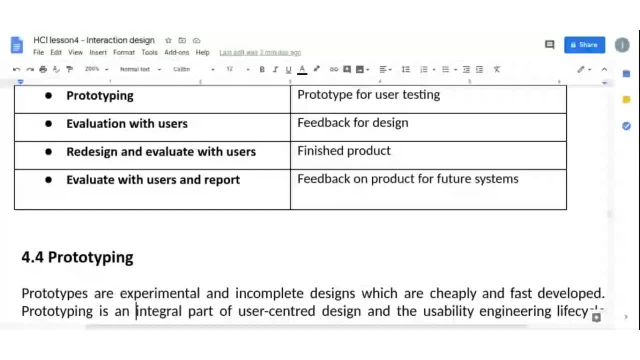 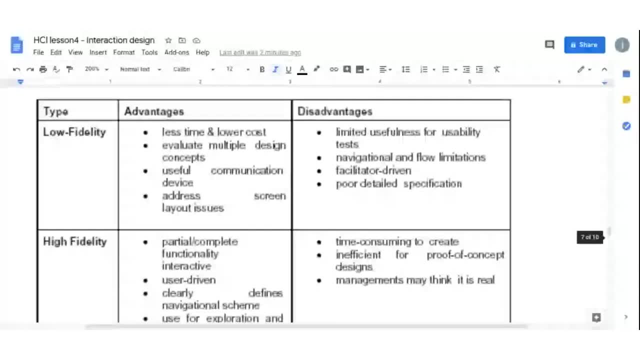 observing. of course, you would like to be asking some questions. when the user does something, maybe you say, now, why did you do it that way? and so that also. so there is this concept of contextual design. contextual design, which is a very important as part of the user-centered design. 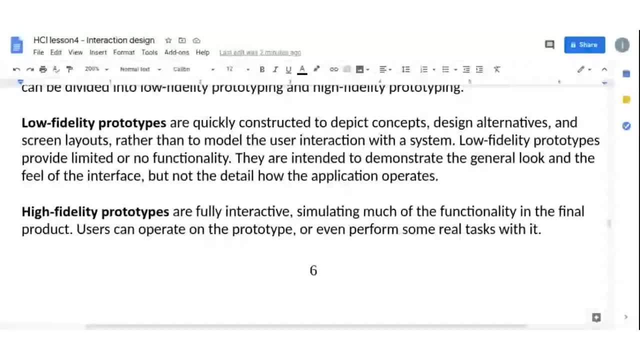 um, so, um, are we better with the audio? is it improving? sometimes, i think, uh, we're having a challenge with the network, so are we still okay? let me, uh, i think at this point it's good to confirm that the audio is still working well. is it still clear? i can see? uh, i'm 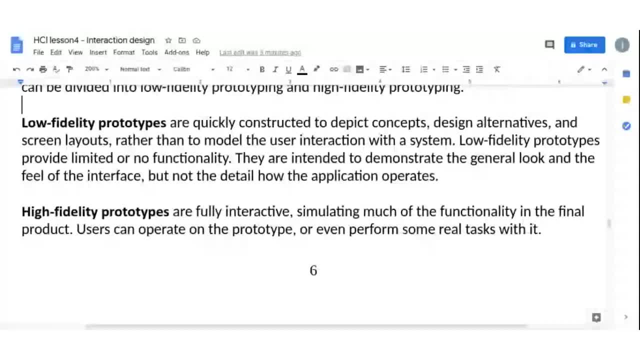 uh, charlo had very, very, uh, it wasn't getting, very, very, uh, it wasn't getting. so, uh, let me have a confirmation. today the audio are still like good and strong. is it still strong? yes, let's see a confirmation. not much clear, so i don't know how good it is, but uh, can you, are you at the study? 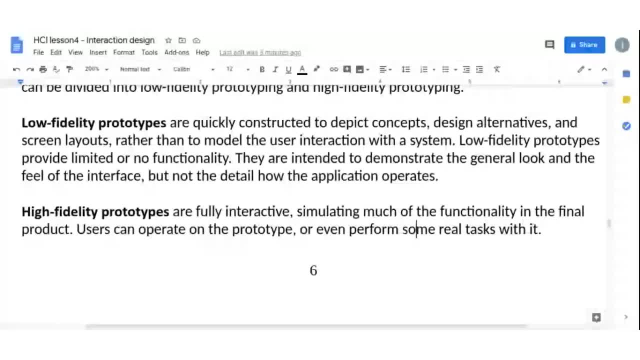 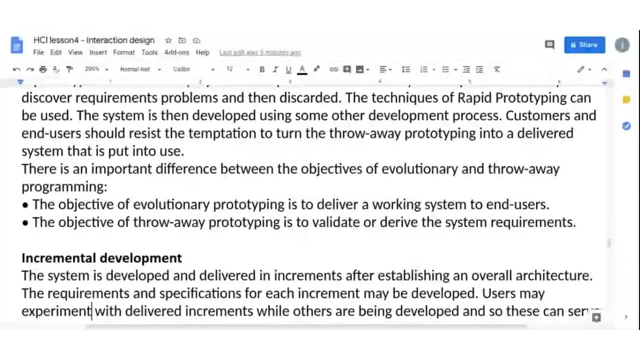 are you at the study? can you? are you at the study? are studying some of the concepts as i share them out. so it means that we are having a challenge sometimes. the network is not very good at the moment and that's actually why we noticed that the, uh, the, the, the document took so long. the document took so long to 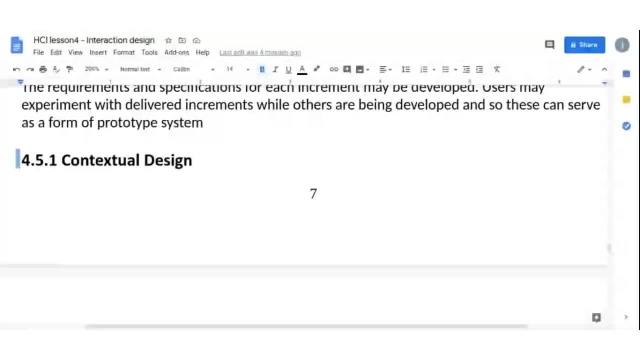 uh to load up was a showing that something is not very strong and of course, in this case it's a the uh. the problem is a networking. my internet is not very strong at the moment, um, so not clear uh, but uh, so let me know, is it? but are you able to follow the discussion? 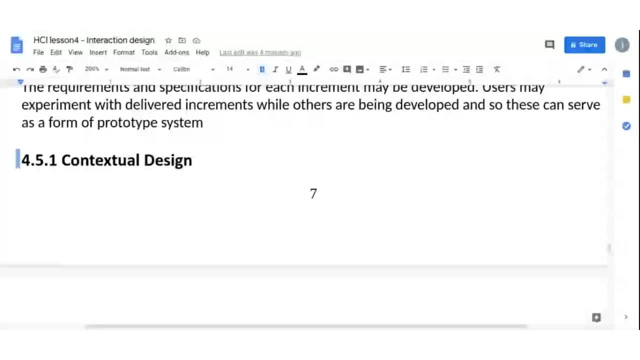 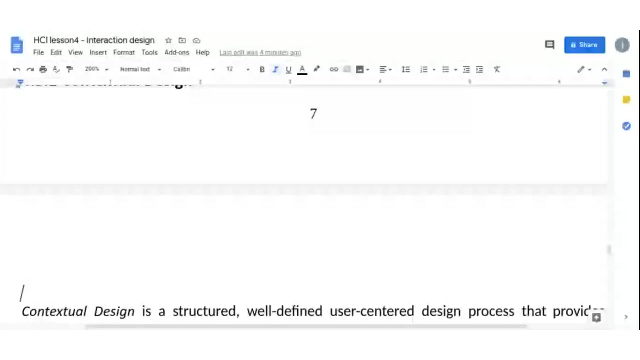 are you able to follow the discussion? are you able to follow the discussion so that we see, if it is too bad, then we uh, we see what to do, so that we see, if it is too bad, then we uh, we see what to do, so that we see what to do. 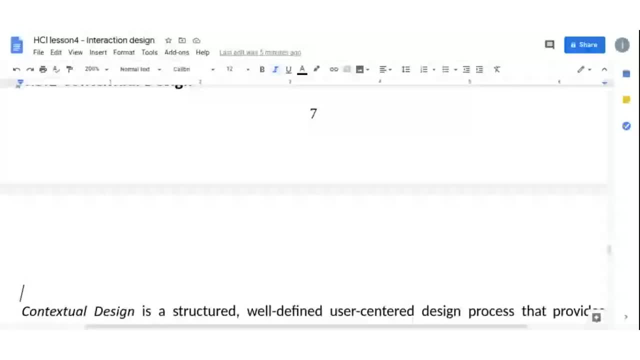 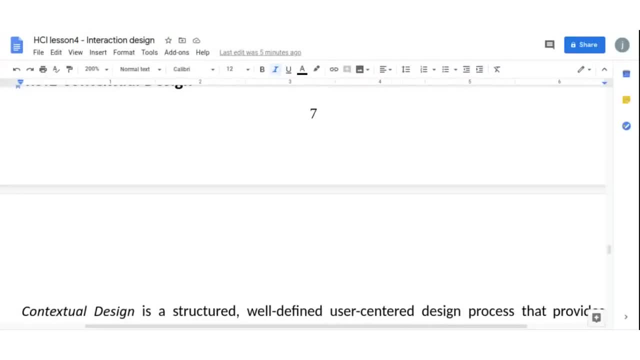 what I will do is that I will not keep us for long, So let me just share a few more concepts, and so we will not take, I will not delay it for too long, because we don't want to continue for too long with that. Well, Innocent is saying, you can follow the discussion. 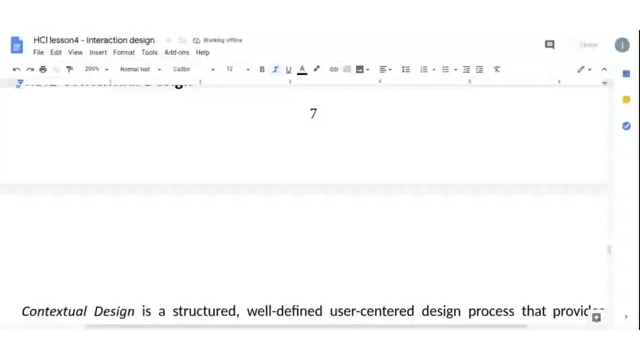 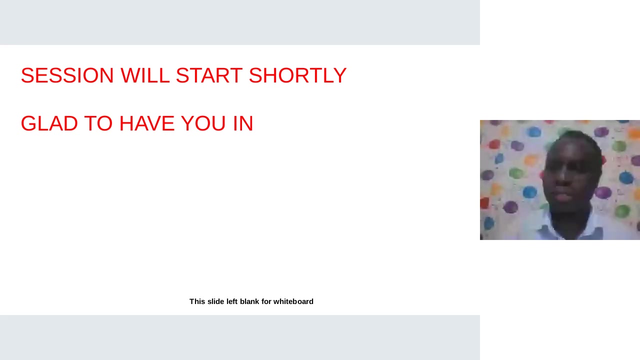 That's good, Thank you, That's encouraging. So, as I said, I will not take too long, So let me begin. I remember I have one more area that I will just raise, but again, it will take a very, very short time because we don't want to. All right, Sorry, I think the document is. 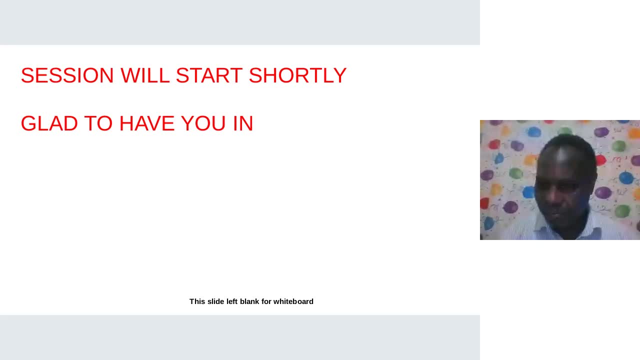 not sharing, So let me share it again. I think I may have touched something on this other end. So let's see, Let's try to. let me try to share the document again And hope it do not take too long, So, but otherwise. so we are talking about the contextual. 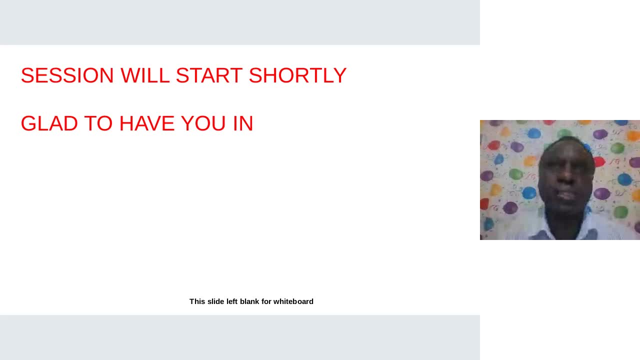 design, the concept of contextual design, So let me just try to share it again. So we are talking about the material side of the room And, as I said before, I will leave it atÖ. See that I also said that somewhere the incidents can also have related society. 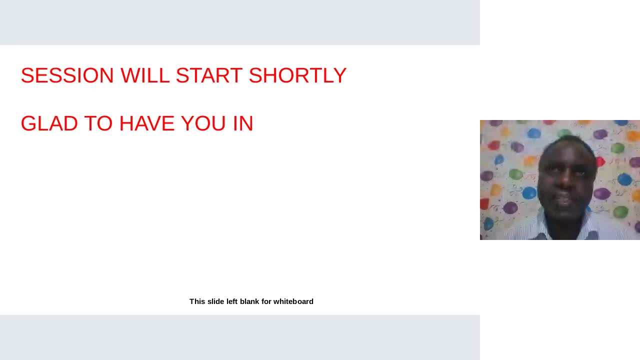 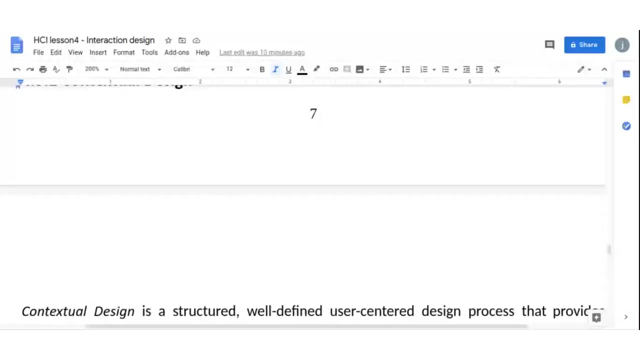 not necessarily the hissing of government. Absolutely, Was I. you know, it's it toShouldá The one that is. I think that is most important is that cutting down on the teacher représents Only the teacher. Yep, She sounds Excellent. Yeah, That, Gene, you said she knows you as well. Yeah, So we will just try to understand Nene center design as it relates to the center design. It's a main feature there is that it's good, So is part of the user centered design that you also go on there, you, you will gather more data about the user devawing and how the user works, trying to improve your design. 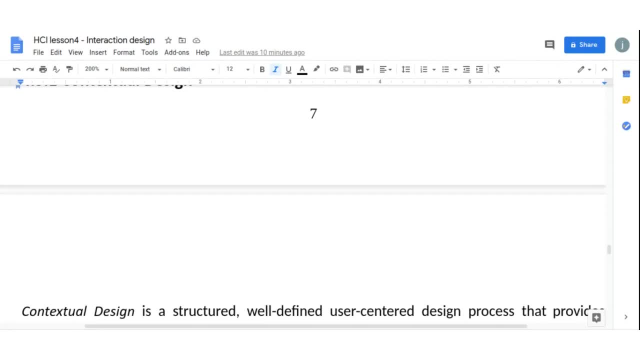 you also do what we call gathering data. that is the whole issue about contextual design, and so for that one, I will let you read a little more and capture the description and discussion involving that about contextual design. well, this is something that is important. why involve users? and so it gives some reason, good reasons to us just to. but there should be more, but these two. 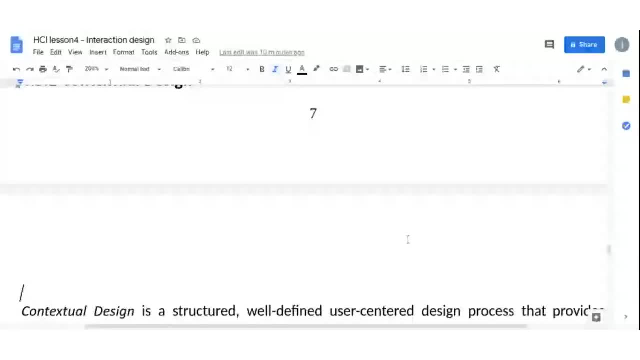 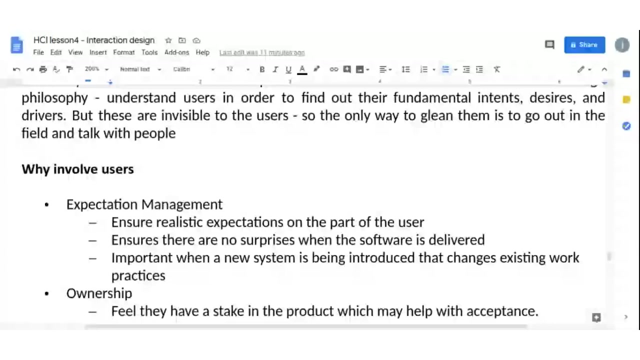 are the expectation. today there is something we are calling expectation management. so what is the user expecting now? if the user is involved a lot through the process and their phases, then you are dealing with the expectation. so they will not be expecting what is not there, because they have been. 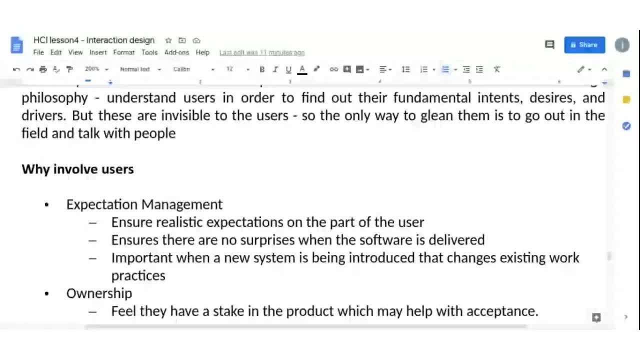 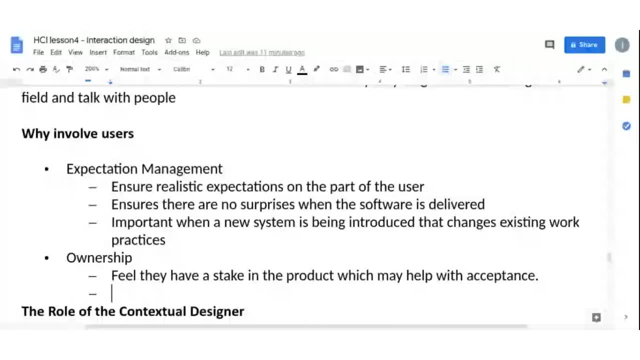 part of it, and so they already know what to expect and also, if it's good, they know that you are winning the user. their ownership, of course. the expectation management is part of the ownership. also, managing the ownership: you want the user to own the process as well as the final product. 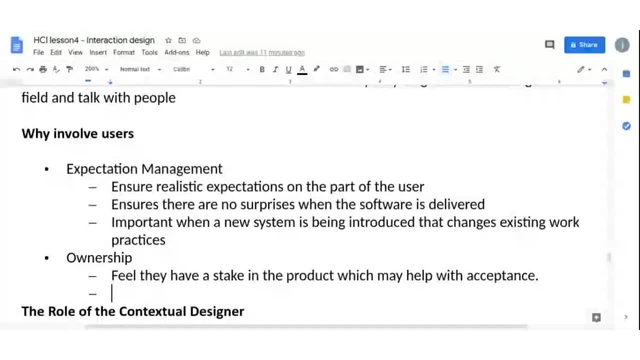 that will come from this. so what is the role of the contextual design? so all these I'll let you look at. this describes a contextual design, the issues that are to be dealt with, how to do the contextual inquiry and related the issues, uh. so all these are. let the student read at your own time, but remember. 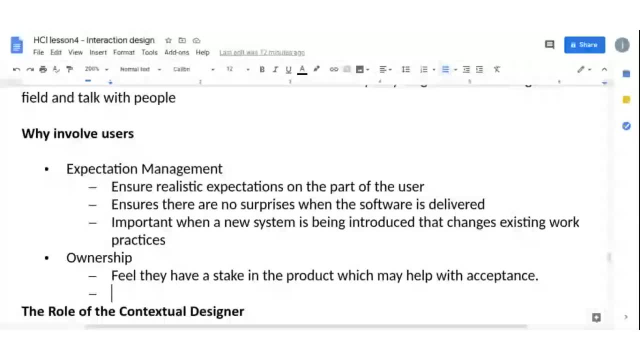 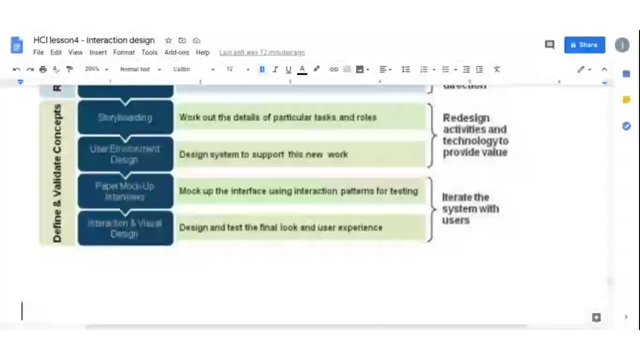 they are important to be understood, but I don't think there are necessarily any complex concepts, concepts within the part that I'm leaving out, So I want you to look at that. Of course, I'm also trying to be sensitive about audio, So it's not good to extend too much when we have that challenge.